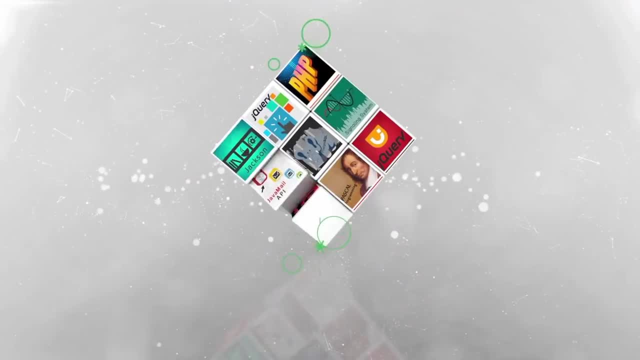 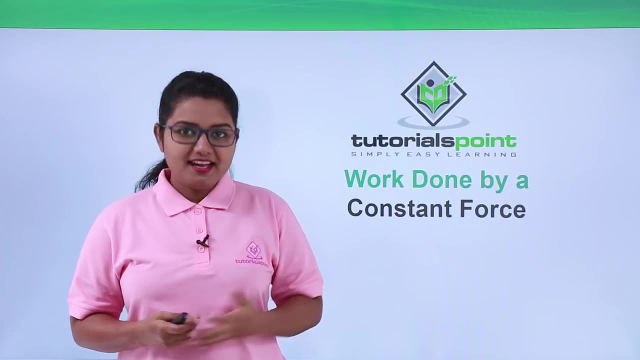 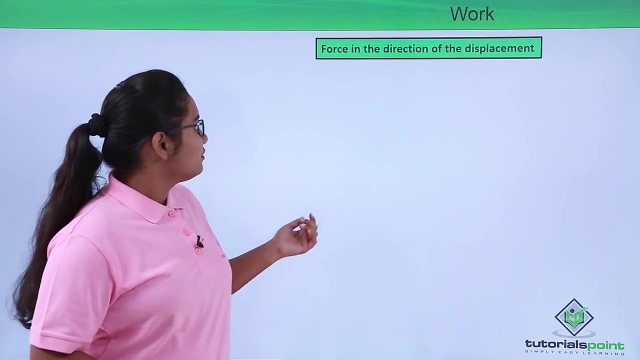 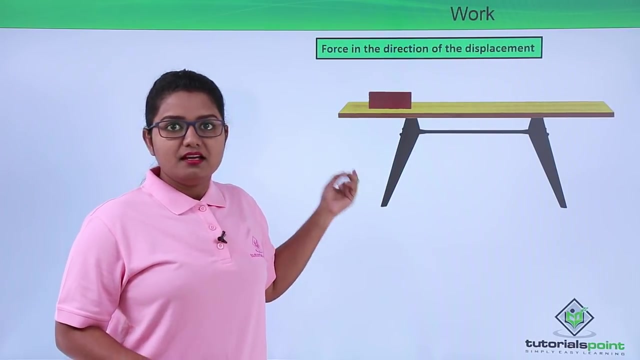 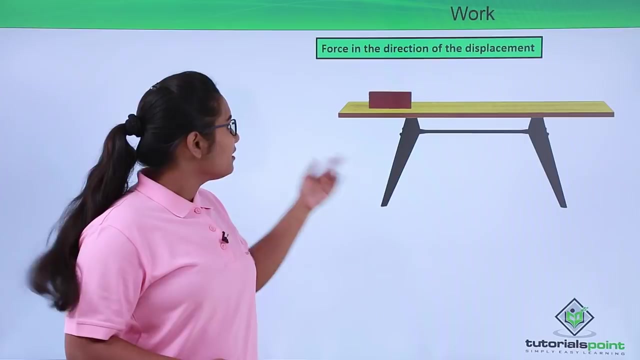 Hello friends, in this video we are going to talk about work done by a constant force. So here, let's say, we have a table and we have placed a block of wood on it. Now suppose we want to put a force in the forward direction. that is that direction. So on doing that, let's. 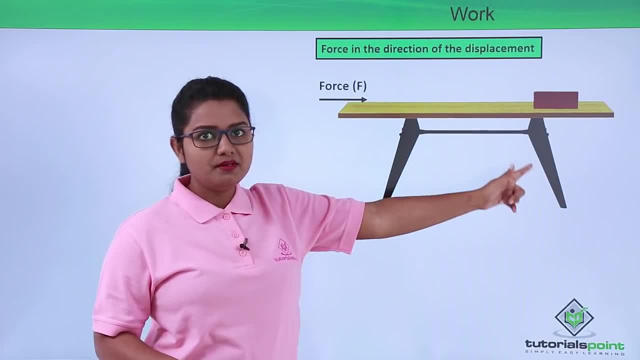 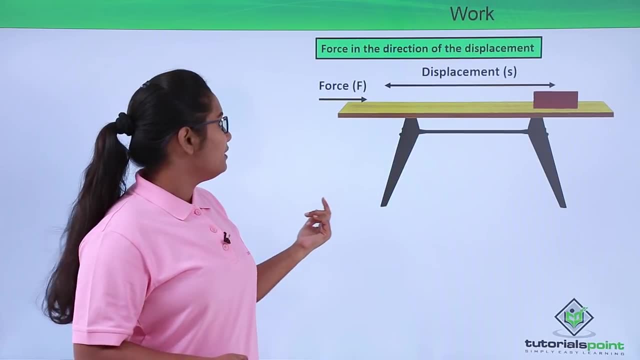 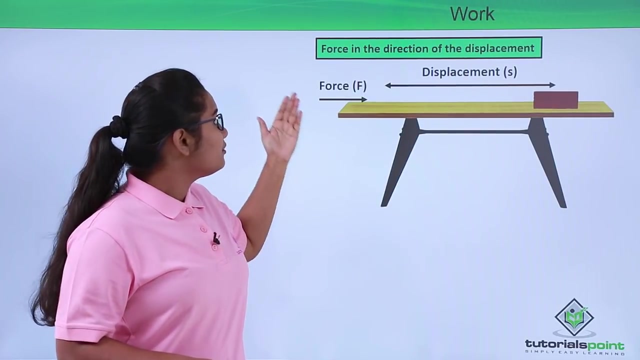 say, the box, the block moves to some distance on the table itself. Now the displacement that the box is covered in this case will be this distance, that is, we have denoted it by the letter S. Now here the force is in that direction, that is, forward direction. 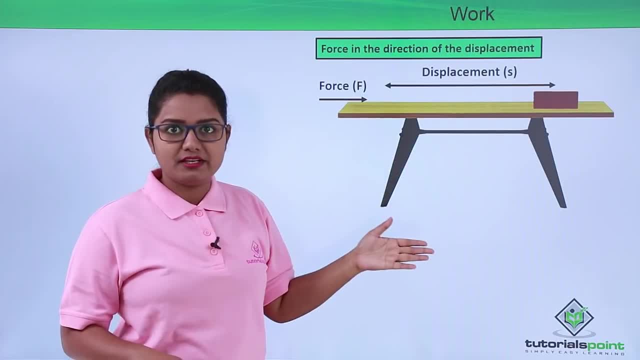 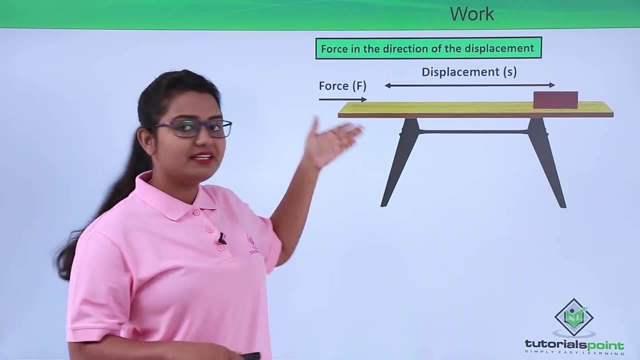 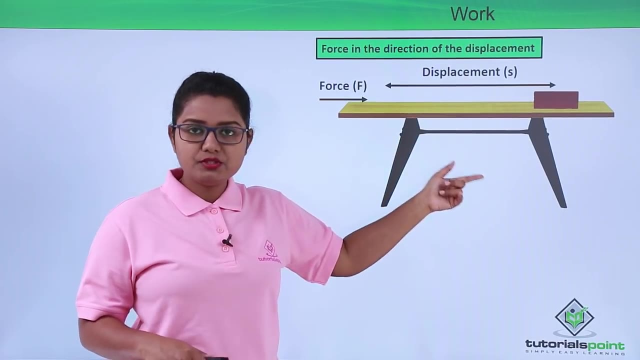 And the body has also moved in the forward direction, which means that the force and displacement are in the forward direction or in the same direction. Now, here there is a force which has been applied to the body, so it satisfies the first condition that we have seen in the 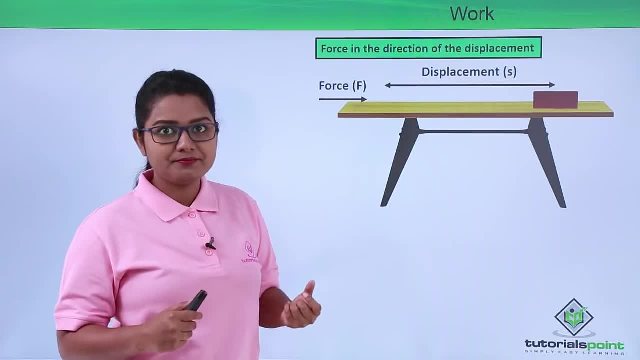 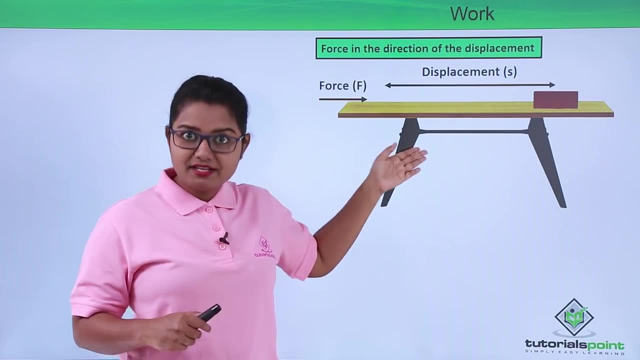 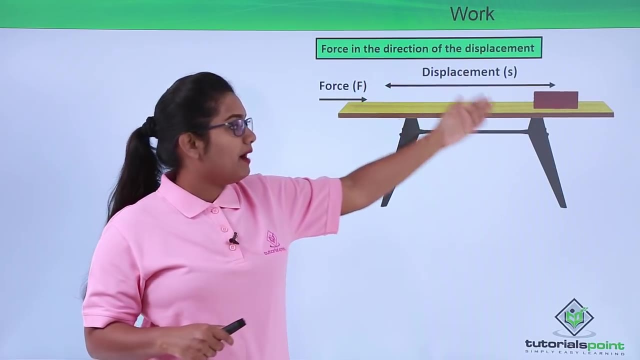 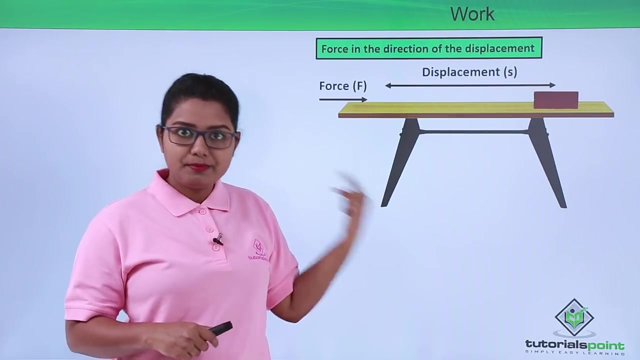 previous video of scientific conception of work, There were three conditions, that is, that the force has to be applied on an object. The second condition is that the displacement has to be made by the object because of the force F. So the object must get displaced. 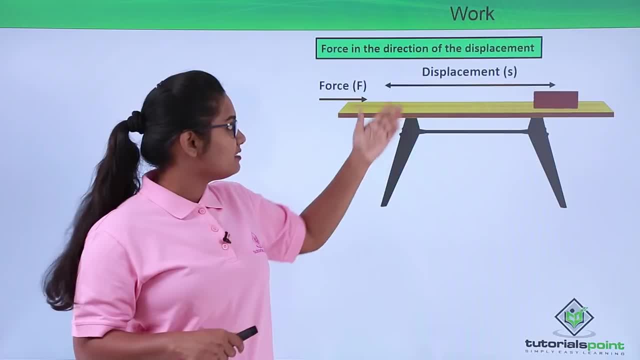 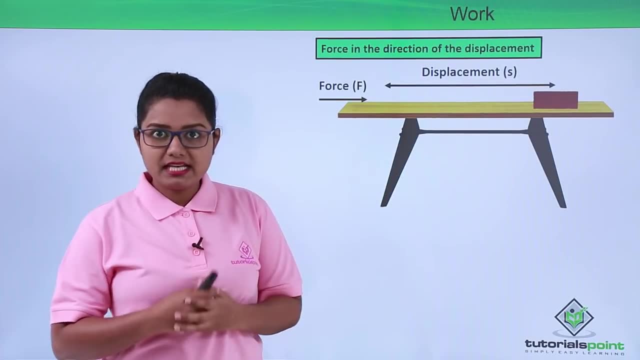 because of the force F. So here, in this case, the force F has caused a displacement S on the block. So the second condition is satisfied. The third condition is that the force has to be made by the object because of the force F. So the third condition is the angle between. 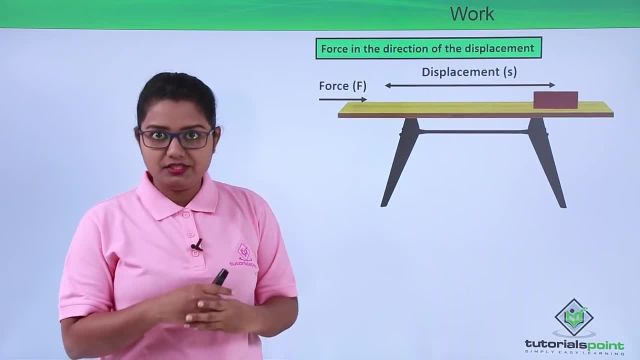 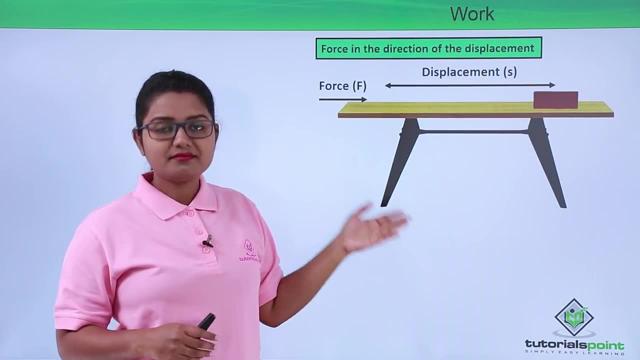 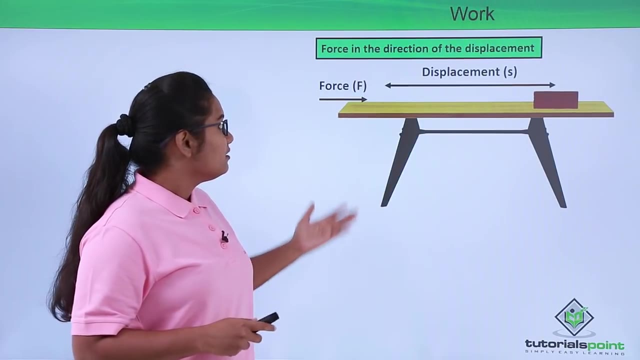 the force and displacement must not be 90 degree. So here we see that both of them, that is the force and the displacement, are in the same direction. So the angle between them is 0 degree. It's not, it's nowhere close to 90 degree at all. So here this activity is. 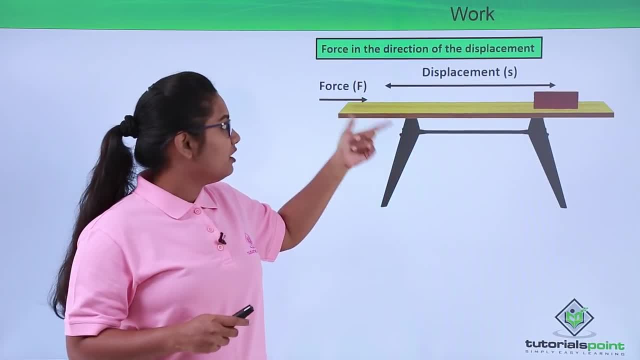 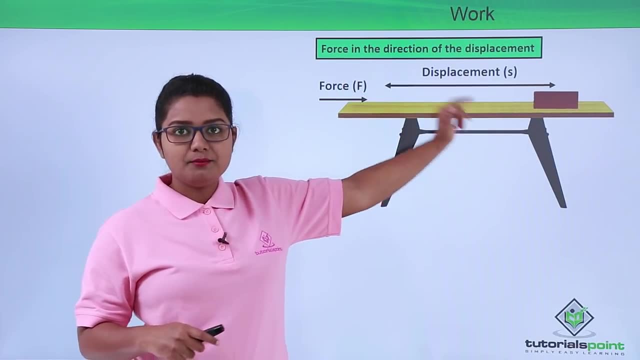 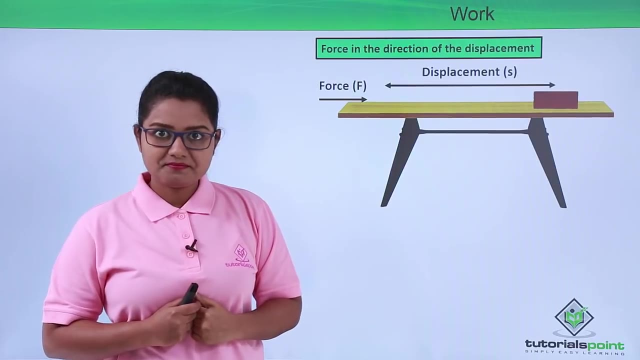 said to be a work, or we can say that a work has been done on displacing the block of wood to the new position by applying a force F. So there has been some amount of work which has been done in this physical activity. Now, the amount of work that has been done here: 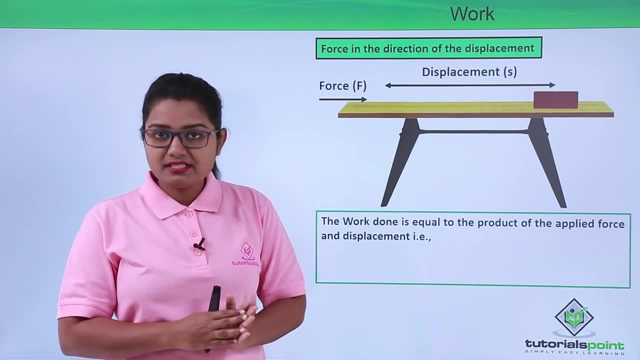 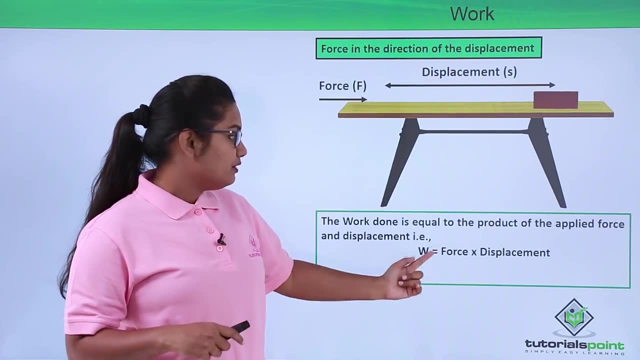 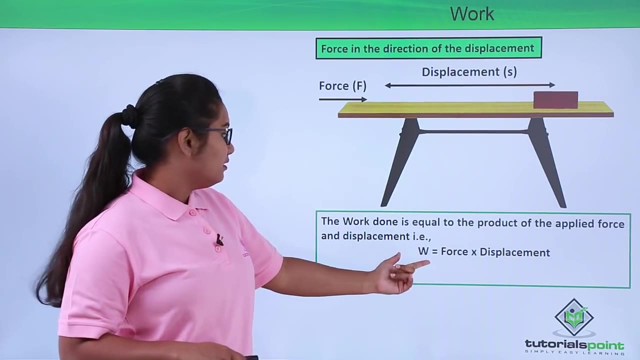 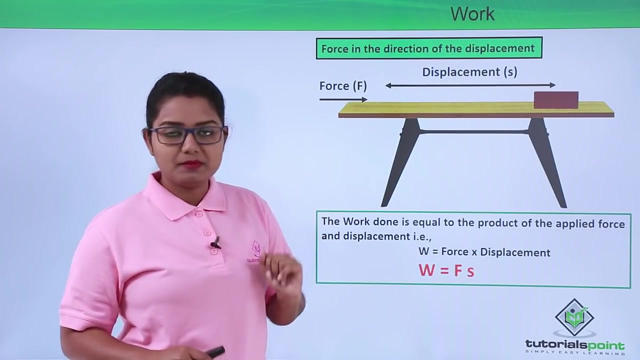 is equal to the product of the applied force and the displacement made by the wooden block. So in other words, W, which is the work done, will be equal to force multiplied by the displacement. so W will be equal to F into S, where F is the force applied and S is the displacement. 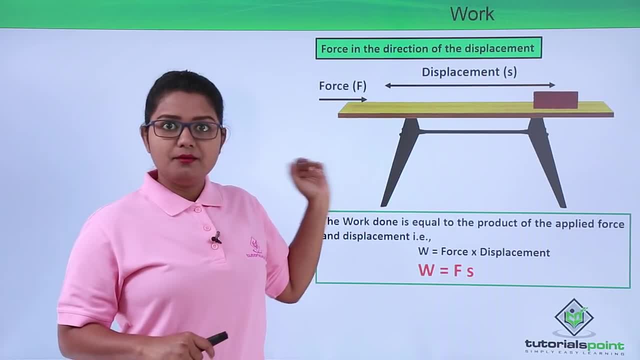 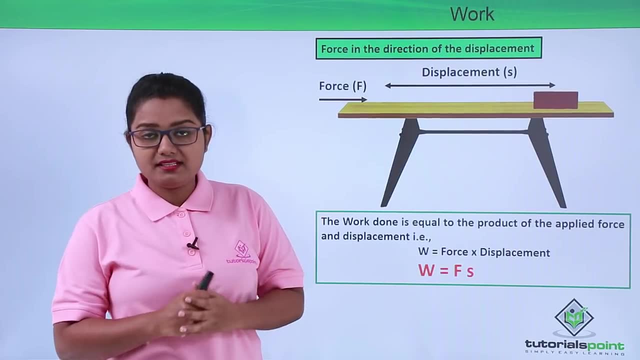 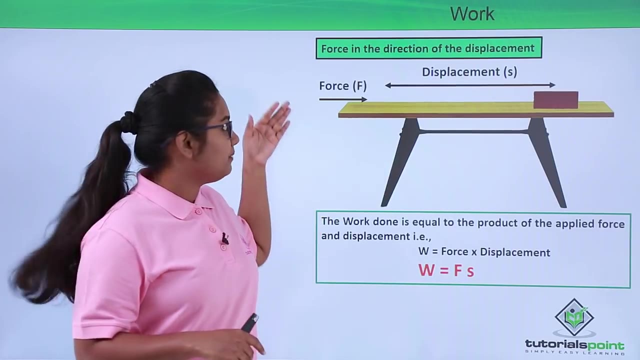 Now we said that this work is the work done due to a constant force. Here the force that we have applied is of a particular value, that is, it is a constant value. It is not changing from time to time. It's a fixed value which we have applied to the block. So we can say: 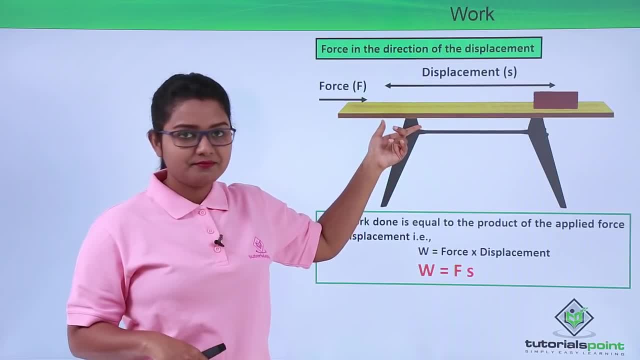 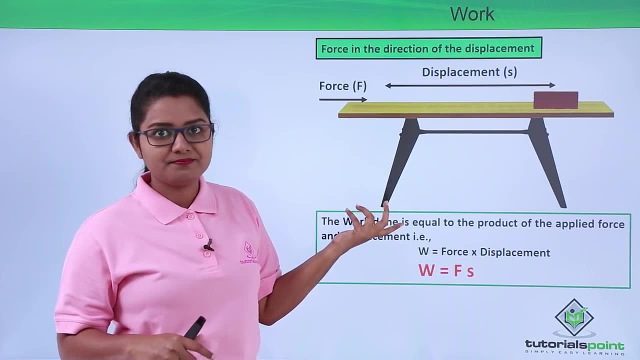 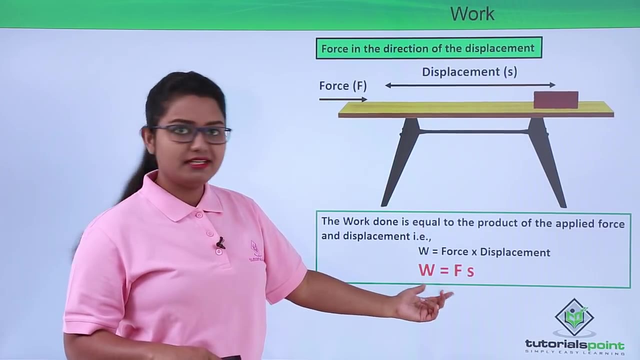 that the block started moving because of the force, So that's why we call it work done due to a constant force or work done by a constant force. Now let us know something more about this physical quantity which we have just now found out. that is work done. 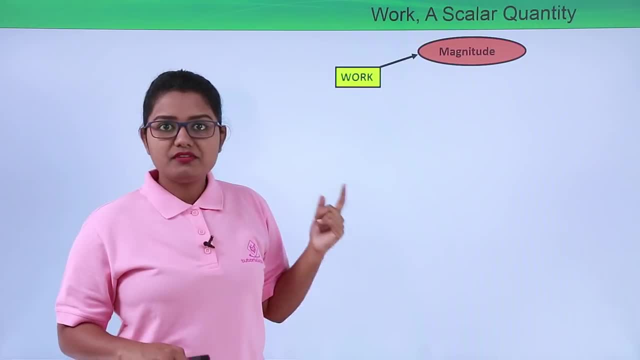 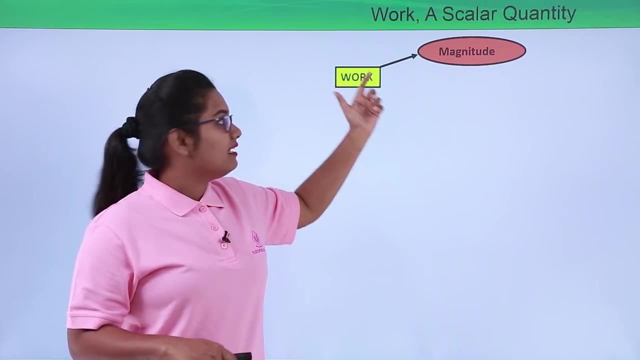 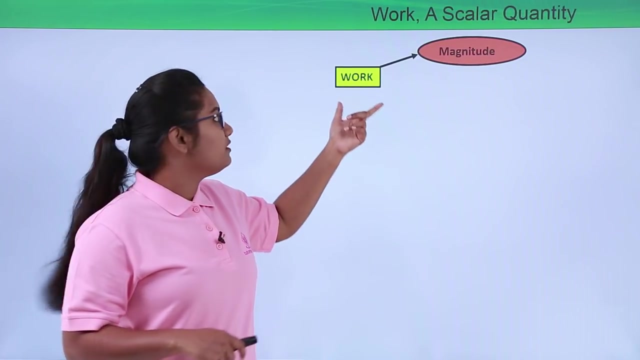 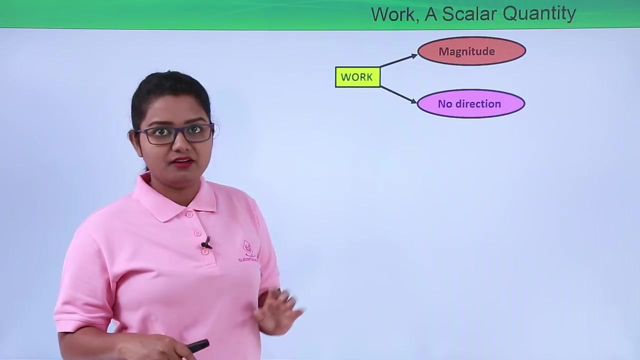 Now, work done in a particular physical quantity, in a particular physical activity has a particular magnitude. It means that it has a particular amount of work that has been done on the body. But this physical quantity work has got no direction at all. It is just an amount of something. 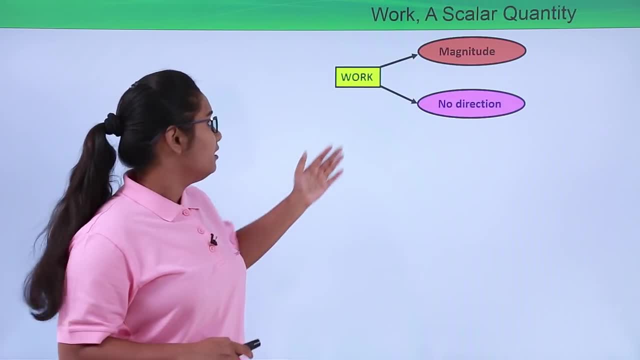 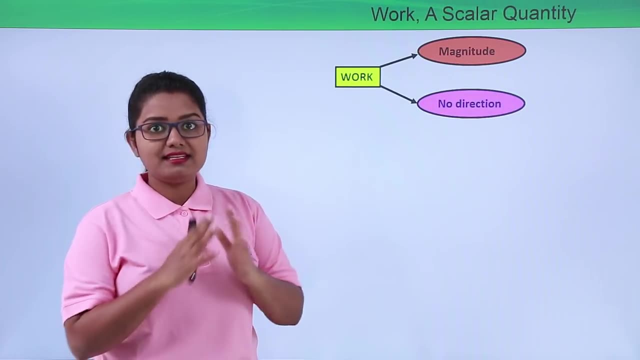 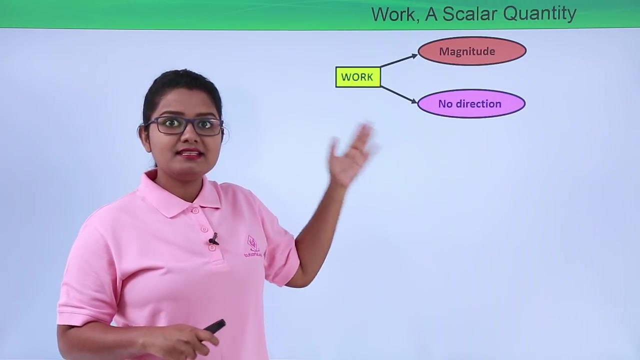 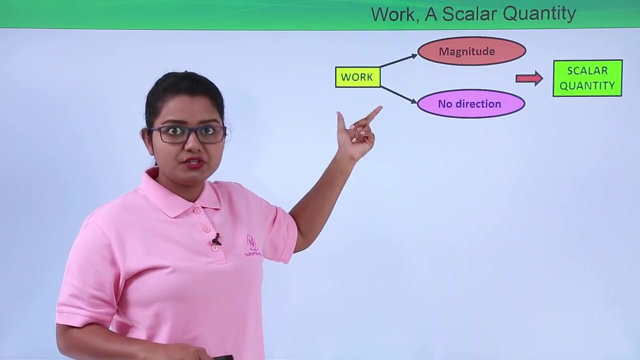 or an amount of work. So we know that any physical quantity which has magnitude but no direction is set to be a scalar quantity. So here, this physical quantity which is work done is a scalar quantity. now let us find out what is the unit in which we can measure this physical quantity. so let's say force be 1 Newton and 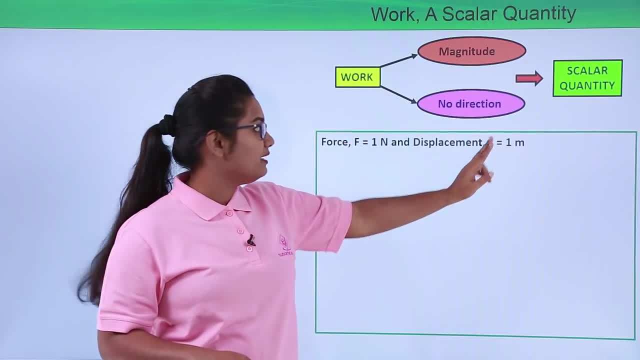 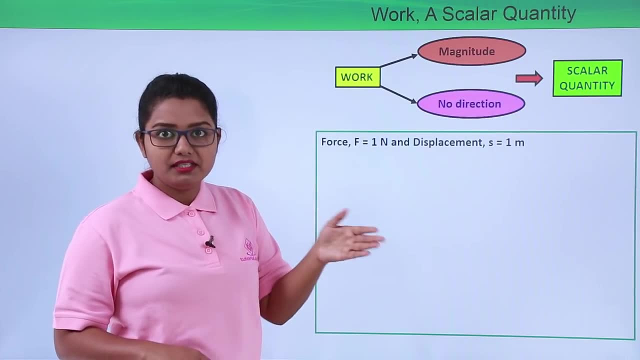 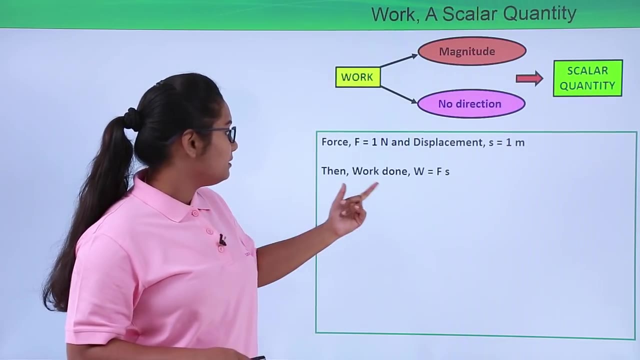 the displacement caused by this force, let's say it be 1 meter. or, in other words, we can say: if let's say, there is a body to which we apply a force of 1 Newton and, as a result, the body moves a distance of 1 meter, now in that case, what will be the work done? work, 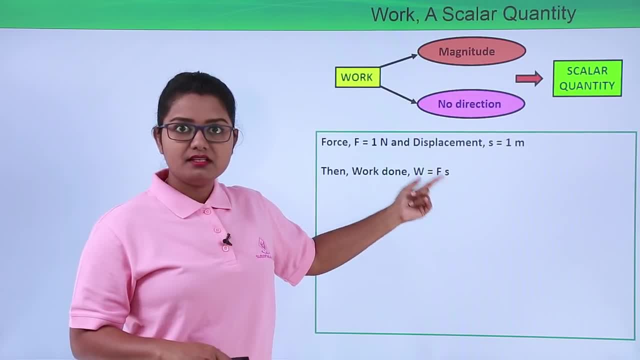 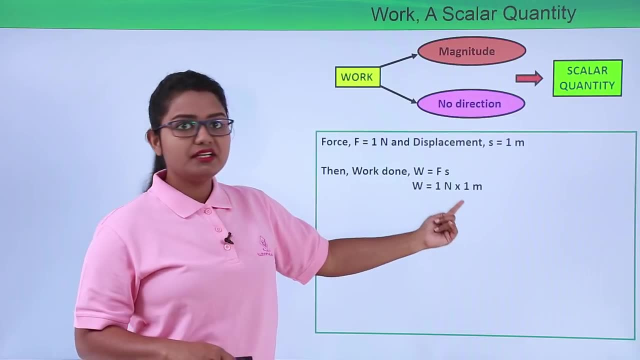 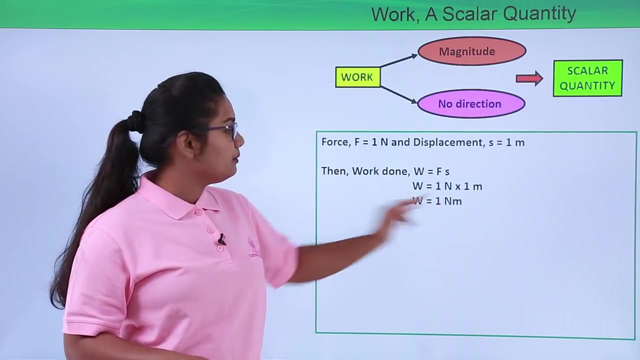 done will be: W equals F into S. here F equals 1 Newton and S equals 1 meter. so W will be equal to 1 Newton into 1 meter, which is 1 Newton meter. now this unit Newton into meter has a particular name, which is called joule. so here the work done will be 1 Newton into 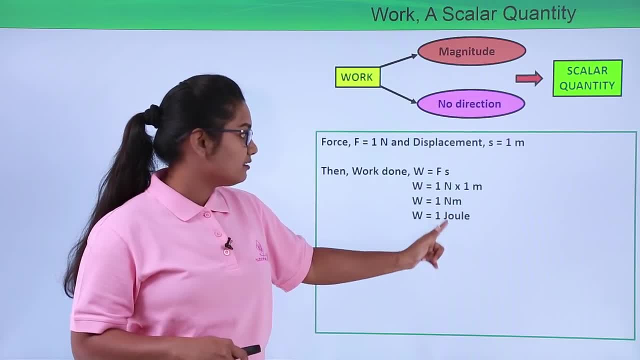 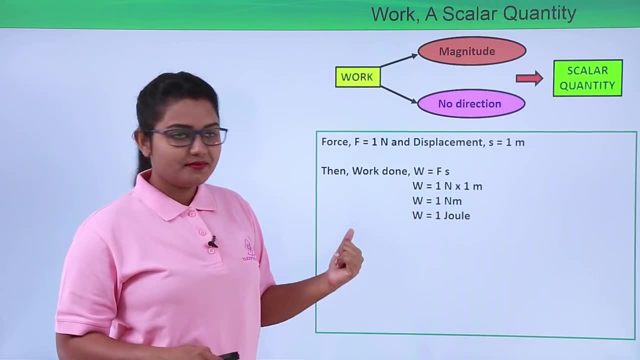 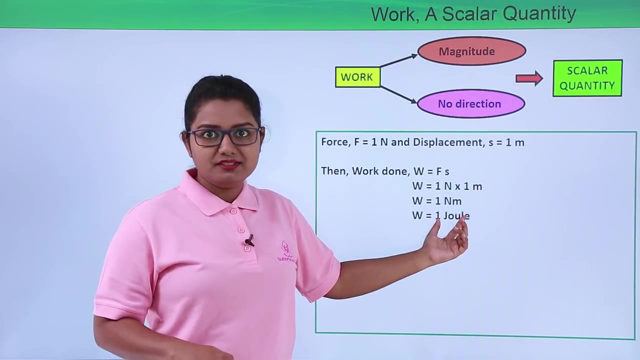 1 meter and the unit of work done is joule. now, this unit is measured in terms of joule, that is equal to Newton into meter. so the unit of work done is joule. now, this word is derived from a scientist, to honor a scientist and whose name was joule. so the unit of work 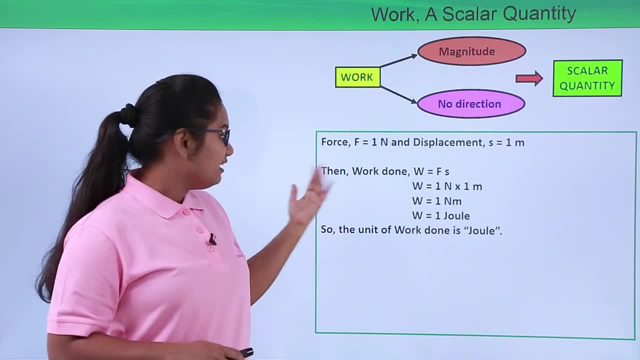 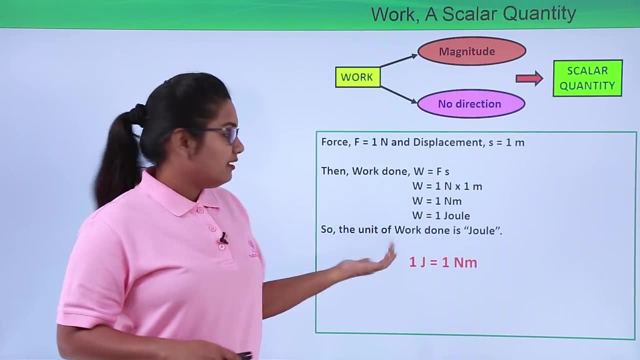 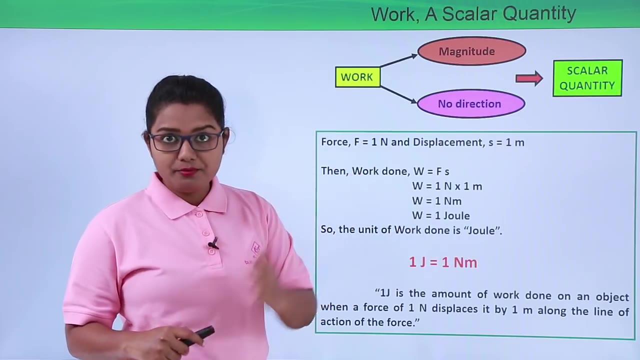 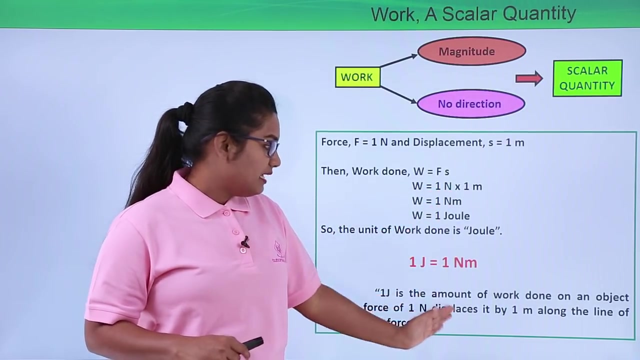 done is found to be joule, so we can also define 1 joule as 1 Newton into 1 meter, that is 1 Newton meter. In other words, we can define 1 joule of work as the amount of work done on an object when a force of 1 newton is being applied to it, which displaces it by 1 meter along the line of action of the force. 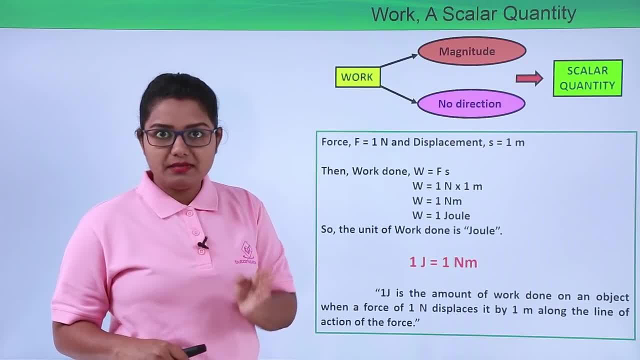 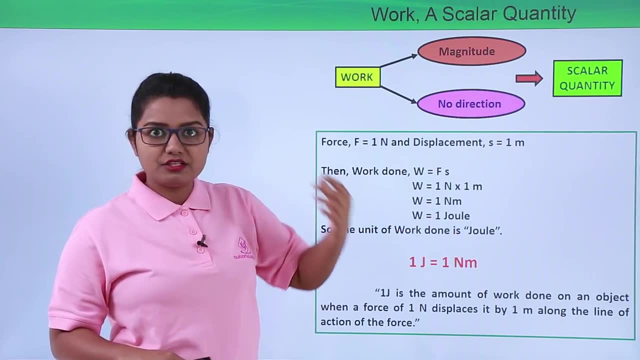 Which means that when 1 newton of force is applied to a body and, as a result, it moves, it gets displaced by 1 meter in the direction of the force- then we say that the amount of work done in that case is 1 joule. 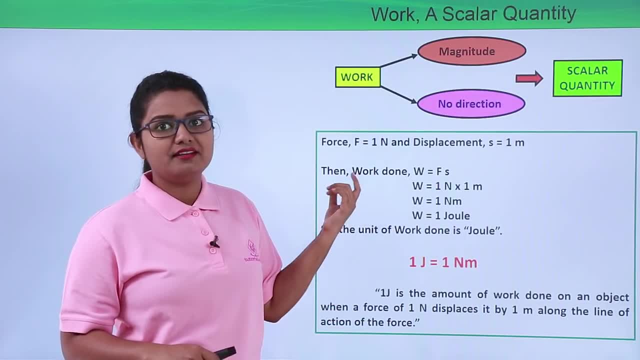 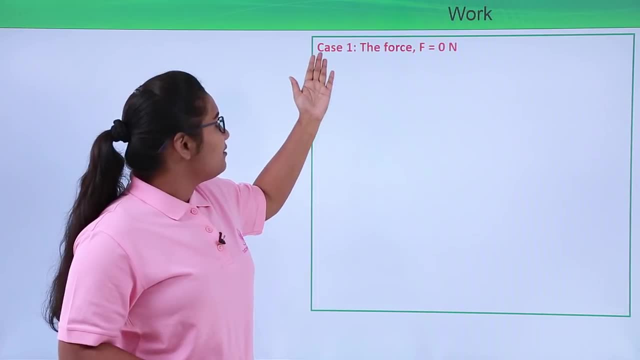 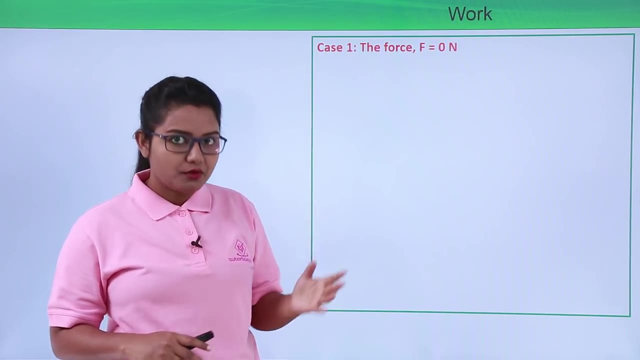 So this is how we define 1 joule of the amount of work done on any object. Now let's say for case 1. Force is 0, that is, we do not apply any force to a body. Then let us see what happens. 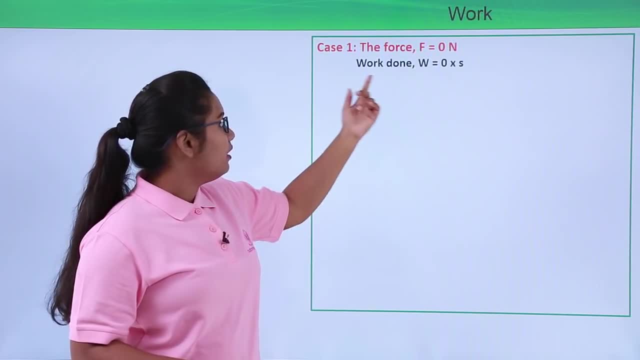 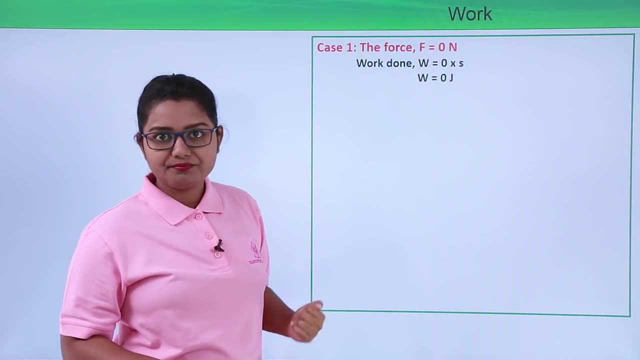 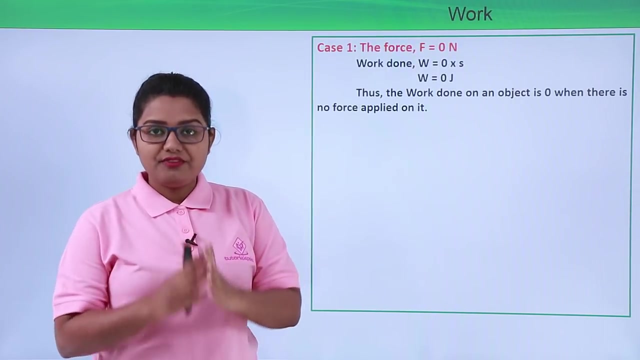 So here force equals 0 newton, So work done will be equal to F into S, which is 0 into S, So work done turns out to be 0.. So here we saw that the work done on an object is 0 when there is no force acting on it. 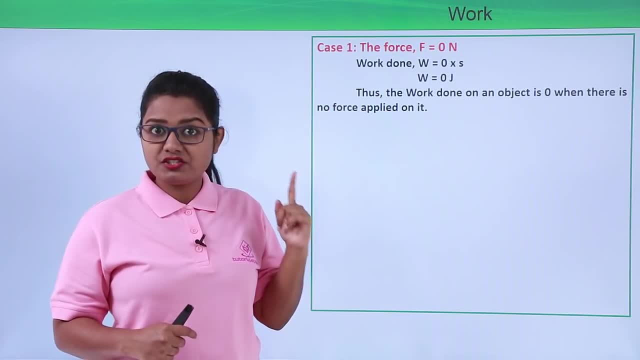 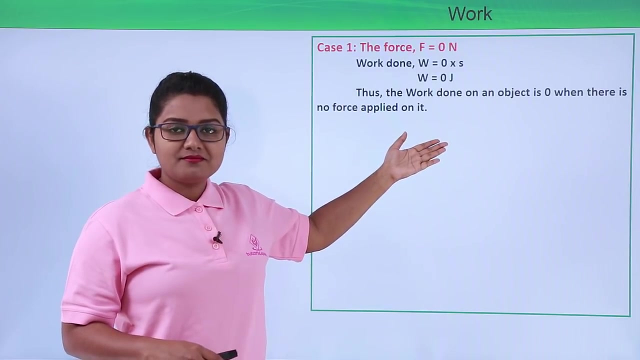 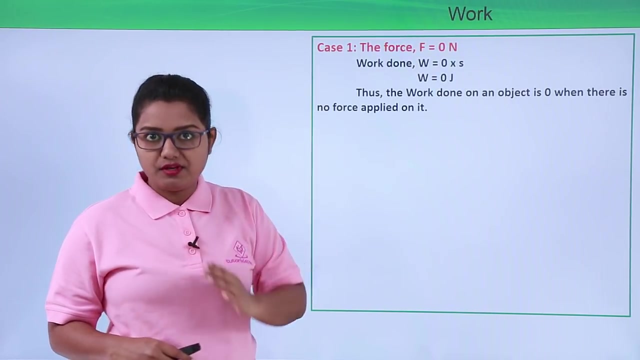 Now this sounds somewhat similar to the first condition of work done that we have seen in the previous video of scientific conception of work. The first condition was that there has to be a force applied onto an object for it to be called as work done or for the physical activity to be called as work. 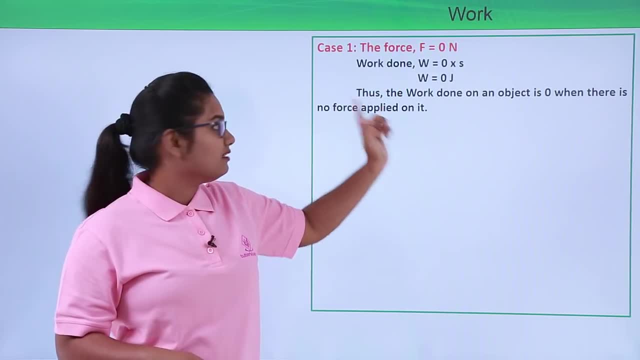 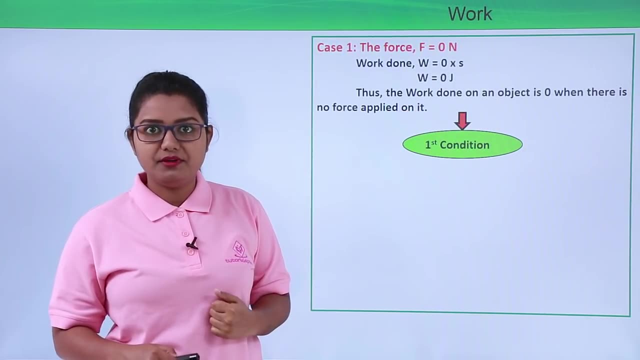 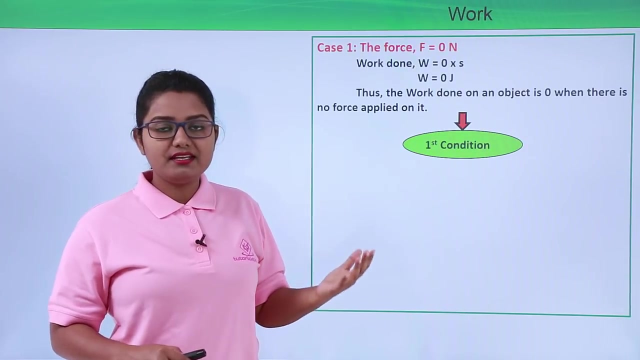 So when there is no force acting on a body, then the work done was found to be 0.. So this verifies the first condition that we have seen in the previous video. Now let us take the case 2 where, let's take, the displacement of the body is 0.. 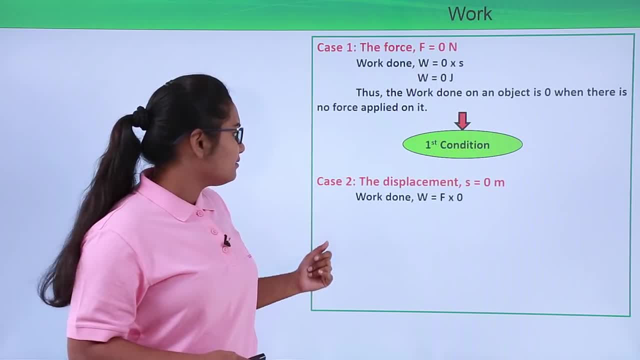 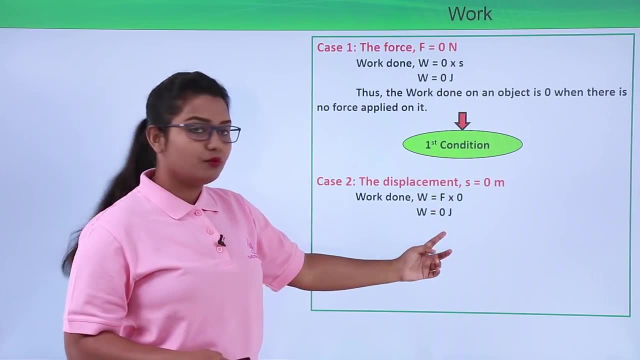 That is, S equals 0 meters. Now, in that case, what happens to the work done? Work done will be equal to W equals F into 0. So this also turns out to be 0. So work done equals 0. 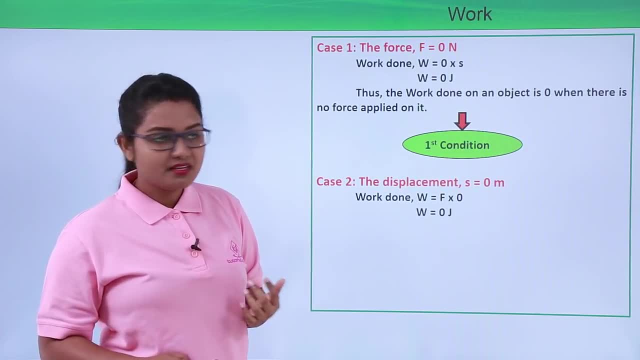 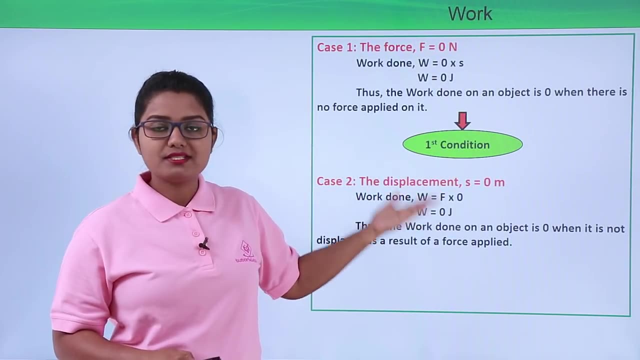 Even when the displacement is 0.. So work done equals 0.. Even when the displacement is 0.. Even when the displacement of the body is 0.. So this means that the work done on an object is 0 when it is not displaced as a result of the force applied. 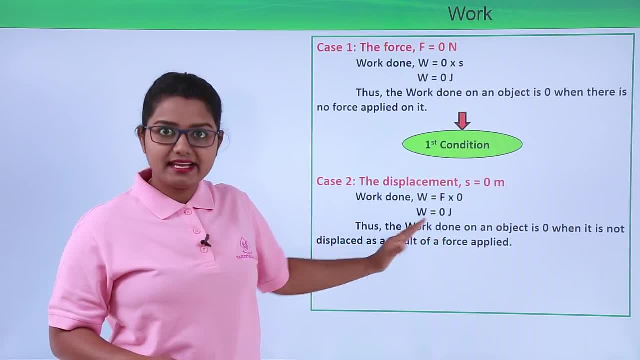 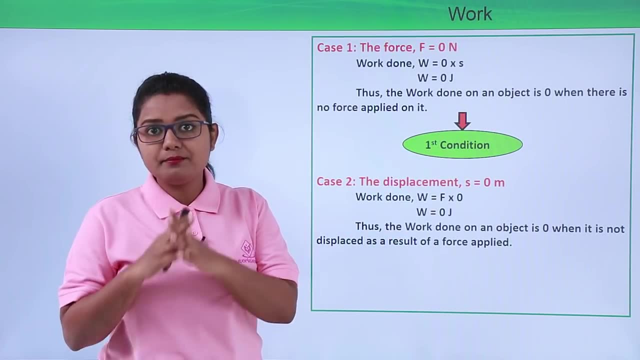 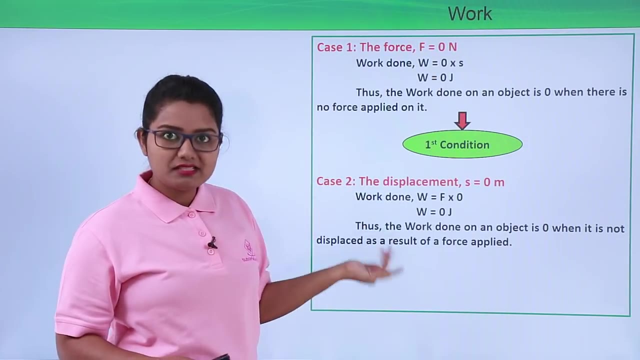 So this is our second condition. put in another way, The second condition was that there must be a displacement in a body as a result of the force. So, as a result of this force, there was no displacement in the body. So the work done is 0.. 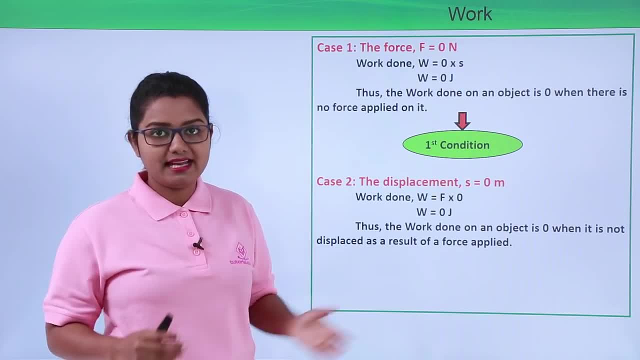 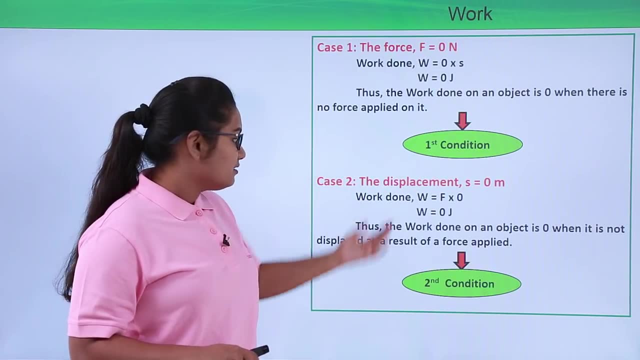 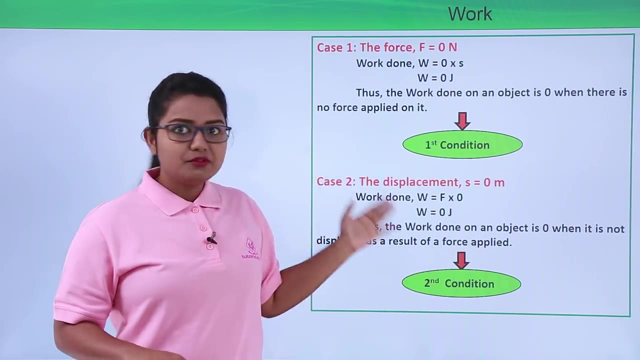 Or in other words, there is no work that has been done on the body when there is a force applied and there is no displacement of the body at all. So this verifies our second condition of work done. So with this, we have come to the end of this video. 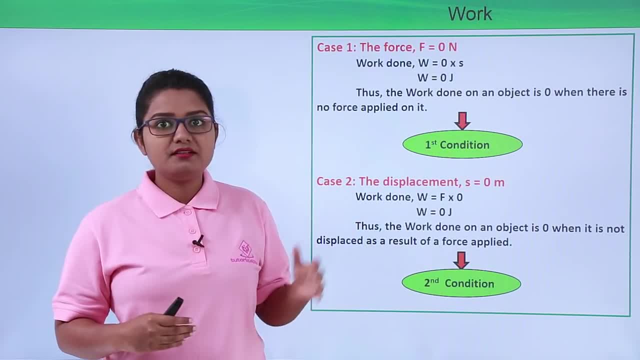 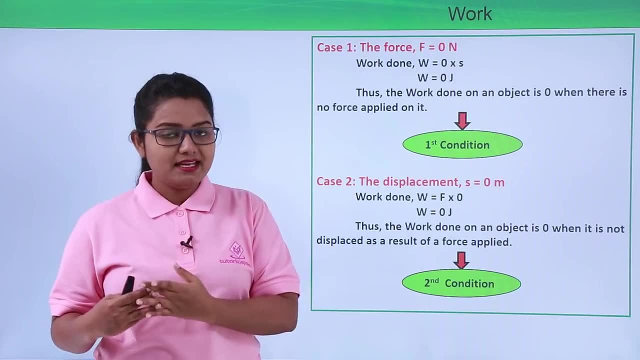 We have learnt in this video about the work done due to a constant force And we have found the formula of the work done to be: W equals F into S And the unit of work done is 0.. And the unit of work done was found to be 1 joule, which equals 1 newton meter. 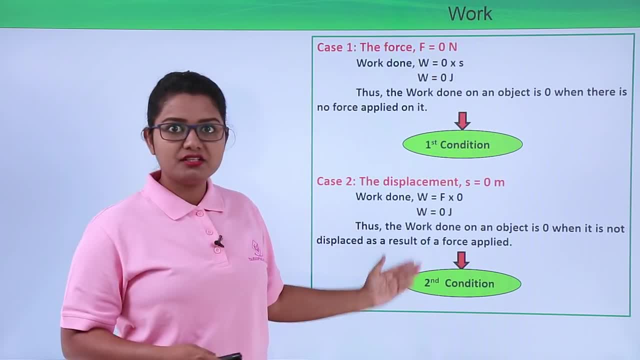 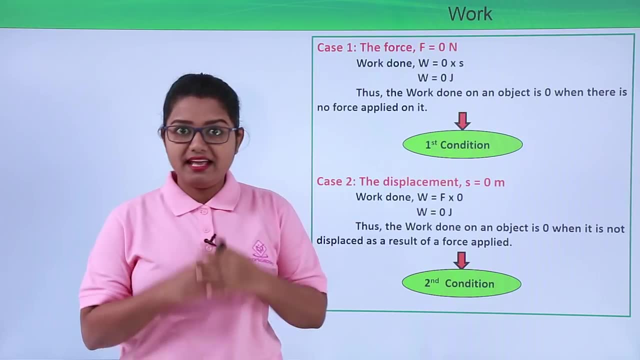 And we have also verified the first and the second condition of work. done So, with this, we have come to the end of this video, And I hope you like this video. Thanks for watching.